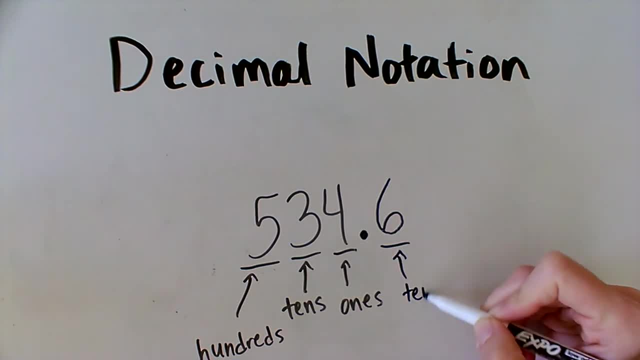 this is the tenths place, So this digit is worth six tenths, and tenths are smaller than ones. They're actually ten times smaller. One tenth is ten times smaller than one, in the same way that one is ten times smaller than ten. Ten is. 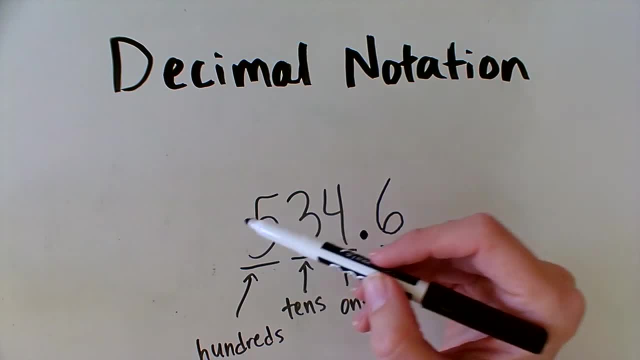 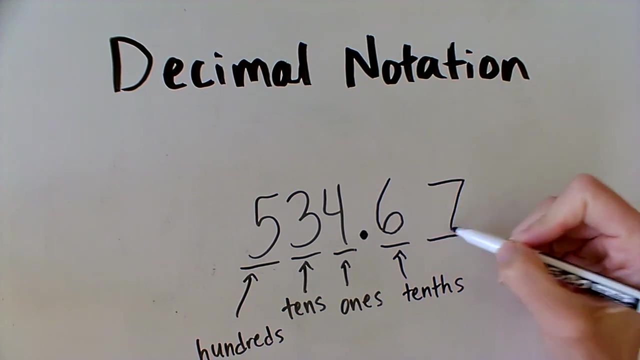 ten times smaller than a hundred. A hundred is ten times smaller than a thousand. That's why it's called a base ten system. So when we move into decimals we're just getting smaller and smaller and smaller. After the tenths place we have the hundredths place. So if I were to put a digit here, I now have. 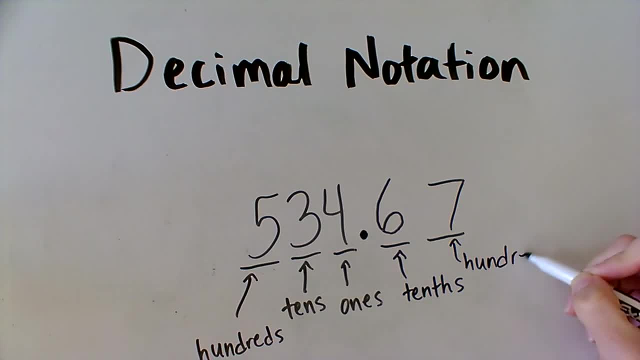 a seven in the hundredths place, so it is worth seven hundredths. Hundredths are ten times smaller than tenths. I could even go smaller. I could put another digit. This would be the thousandths place. but we're not going to do that. 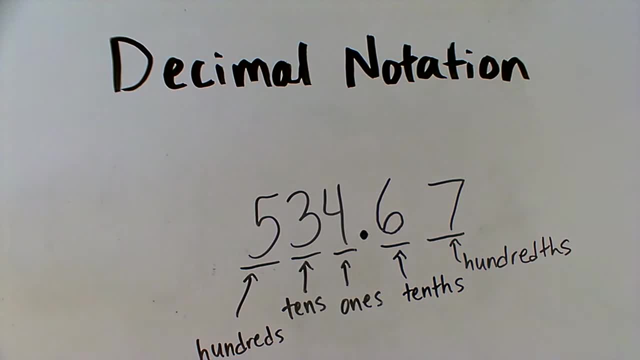 I'm not going to worry about thousandths right now, So if I want to write a fraction as a decimal, I just have to make sure I put the digit in the right place. Let's look at a few examples. Let's try a simple one. We'll start with. 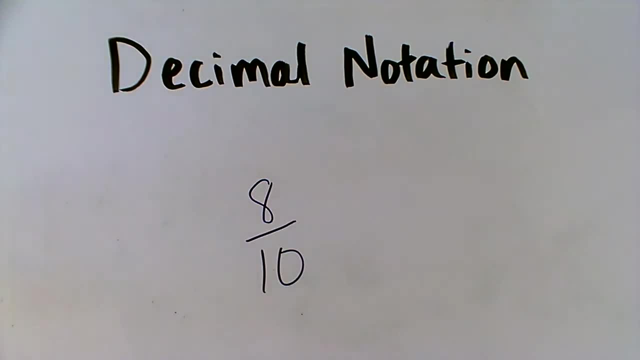 eight tenths. If I want to write the fraction eight tenths as a decimal, I need to put the eight in the tenths place. I don't have a whole number with this fraction. It's not a mixed number. So I'm not going to have anything in the ones place because I don't have any. 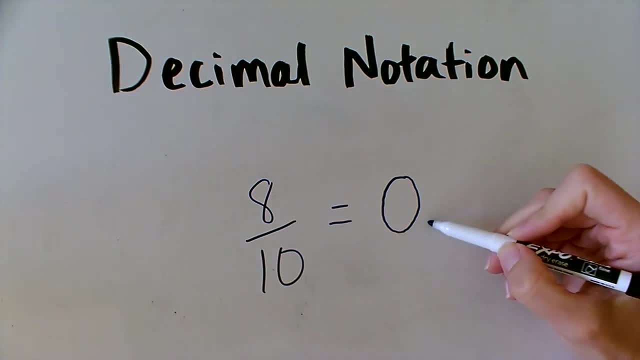 whole numbers, So I have zero. The decimal says: and when you're saying decimal, so I would say zero. and and then I know that the tenths place comes right after the decimal. So if I want to write eight tenths, I have to put the eight in. 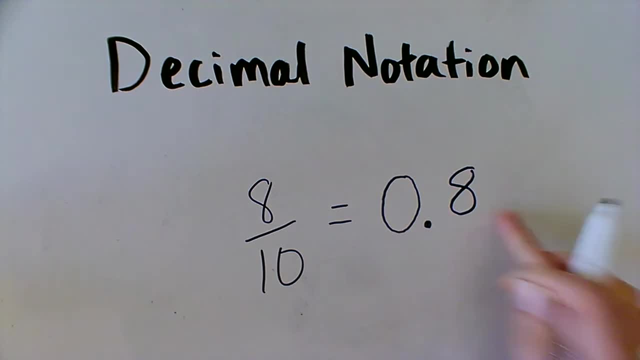 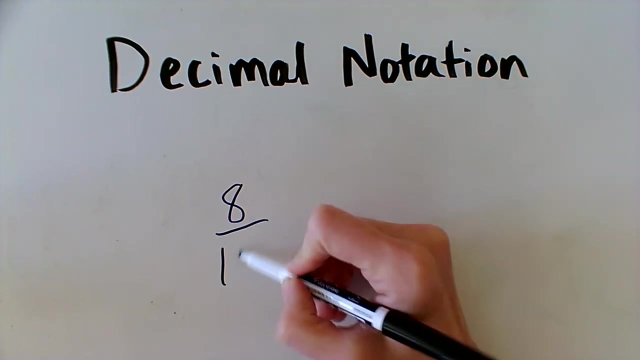 the tenths place like this: This says eight tenths or zero, and eight tenths in decimal. Let's try another one. This time I want to write eight hundredths as a decimal. Well, this time I don't have eight tenths, I have eight hundredths, So I have to make. 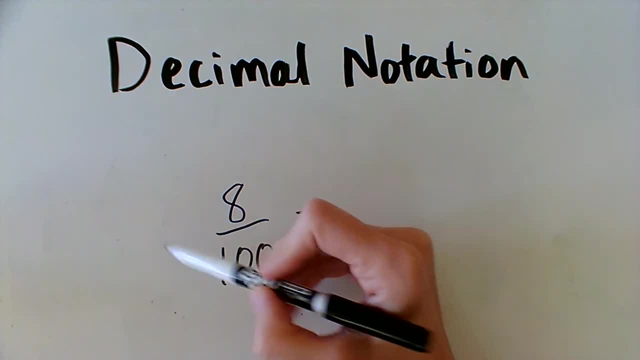 sure that the 8 goes in the hundreds place. Once again, I don't have any whole numbers, so I have zero and I don't have any tenths either. Remember that that 10 hundredths would be equal to 1 tenth. 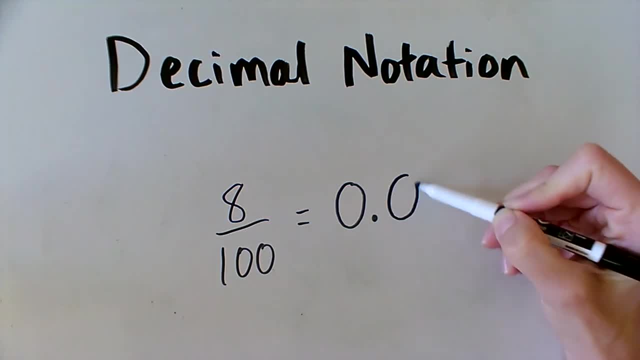 I don't have that many hundredths, so I have 0 tenths, But I do have 8 hundredths. Notice how the 8 ended up in the hundredths place. I needed a 0 in the tenths place as a placeholder. 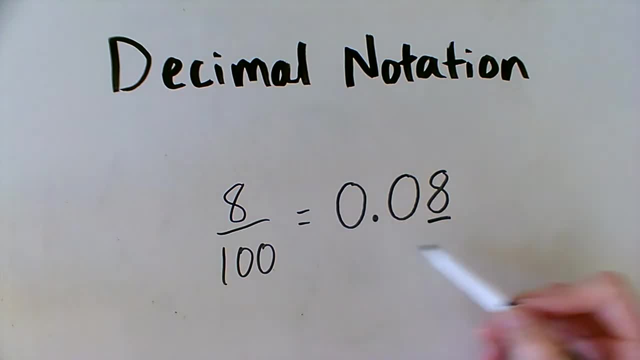 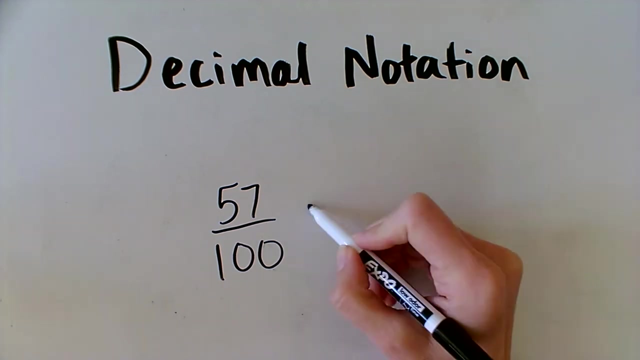 so that the 8 would be in the hundredths place. So this decimal says 8 hundredths or 0 and 8 hundredths. What if I have more hundredths? What if I have 57 hundredths? Once again, I don't have any whole numbers with this fraction. 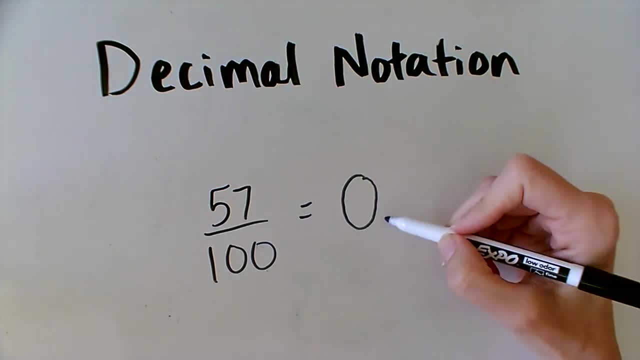 so I have a 0 in the ones place, And then I have 57 hundredths. Well, 50 hundredths, that's actually 5 tenths. 50 hundredths is worth 5 tenths, so the 5 is going to end up in the tenths place. 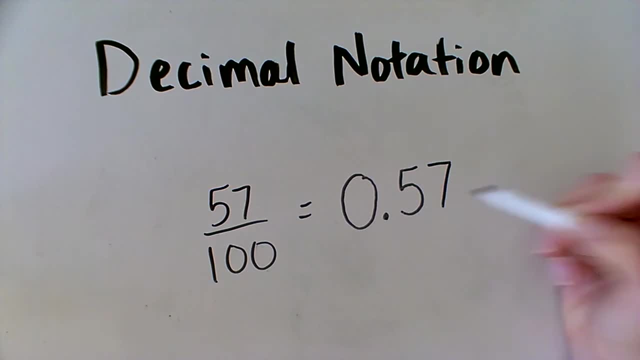 And then the 7 hundredths. 57 hundredths looks like this. I remember 57 hundredths because it looks like the number 57, and it ends in the hundredths place. Another way to look at it is to think about money. 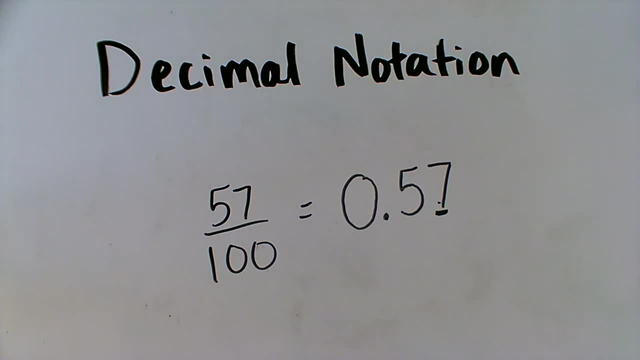 This is how you would write $0.57.. And that's what $0.57 is. It's 57 out of the 100 cents that makes up $1.. Let's look at an example with a whole number. So if I were to write a mixed number, 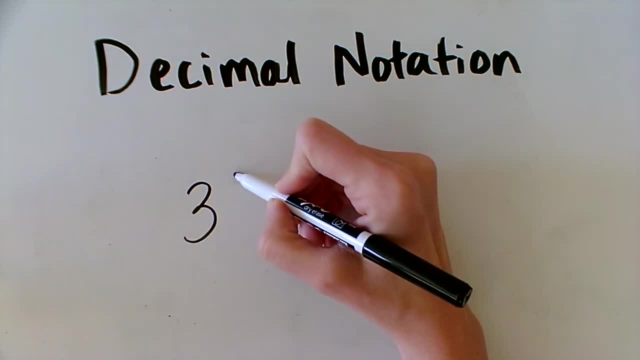 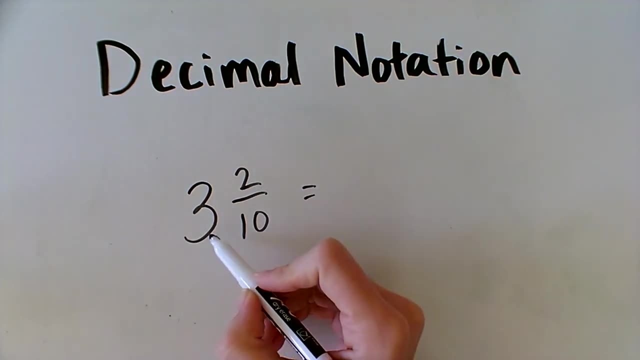 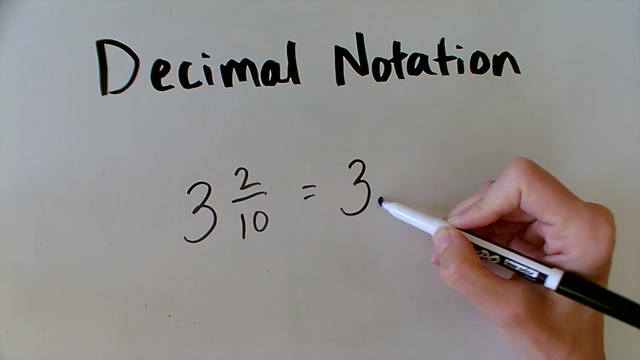 3 and 2 tenths. now I do have something in the ones place of my decimal, The whole number 3, that's worth 3 ones. So I'll have a 3 in the ones place and 2 tenths.